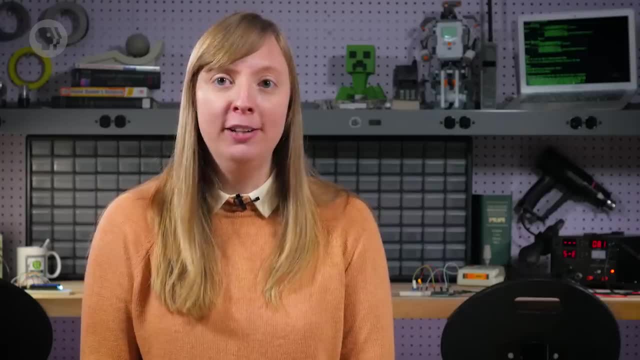 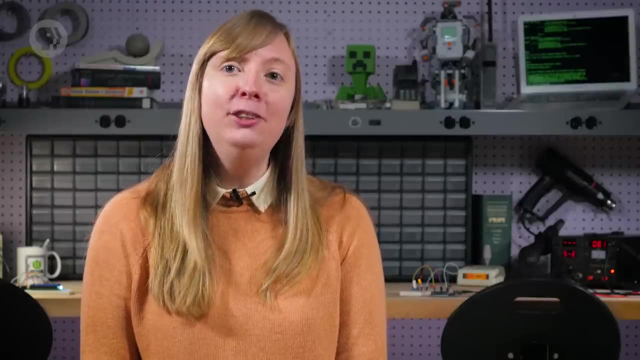 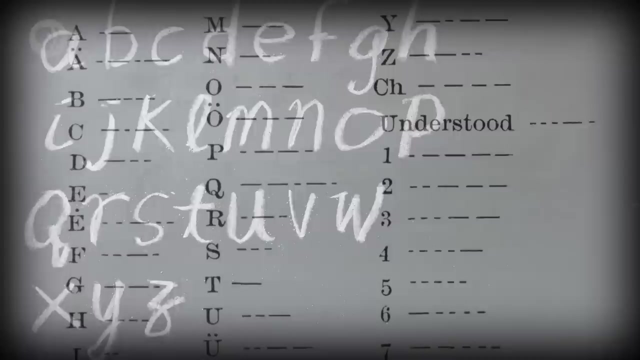 using two different languages. You can think of it like English and Morse code. Hello and mean the same thing: Hello, They're just encoded differently. English and Morse code also have different levels of complexity. English has 26 different letters in its alphabet and way more possible sounds. 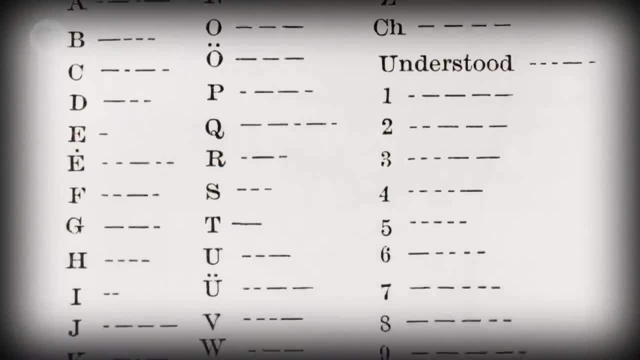 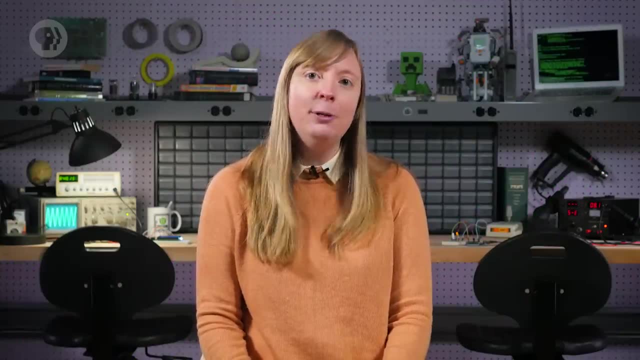 Morse only has dots, Dots and dashes, But they can convey the same information and computer languages are similar. As we've seen, computer hardware can only handle raw binary instructions. This is the language computer processors natively speak. In fact, it's the only language they're able to speak. 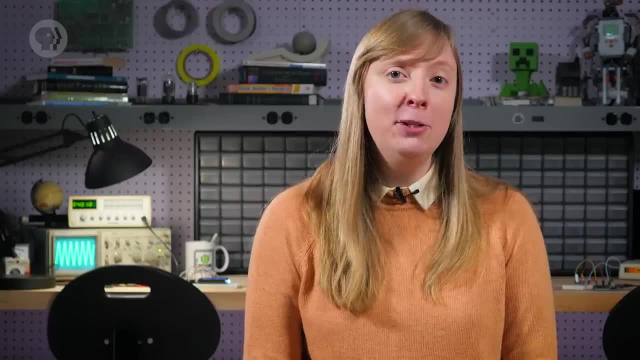 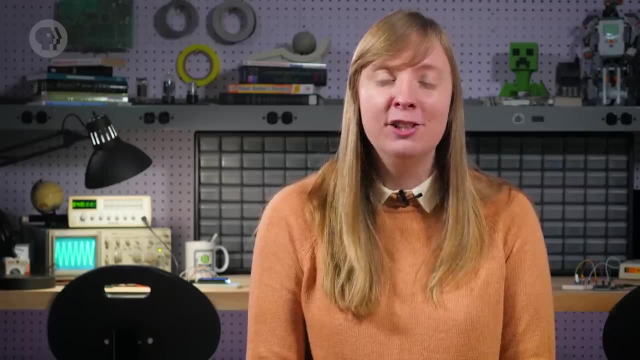 It's called machine language or machine code. In the early days of computing, people had to write entire programs in machine code. More specifically, they'd first write a high-level version of a program on paper, in English, For example: retrieve the next cell from memory, then add this to the running total for the. 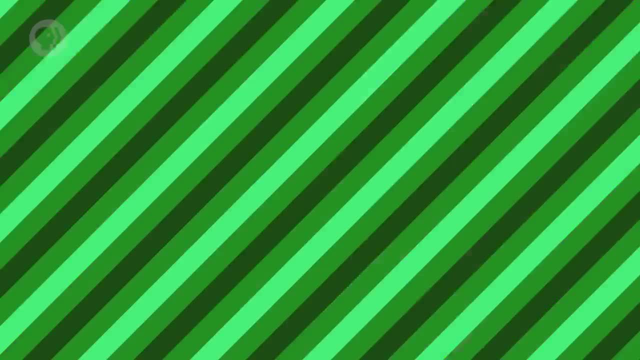 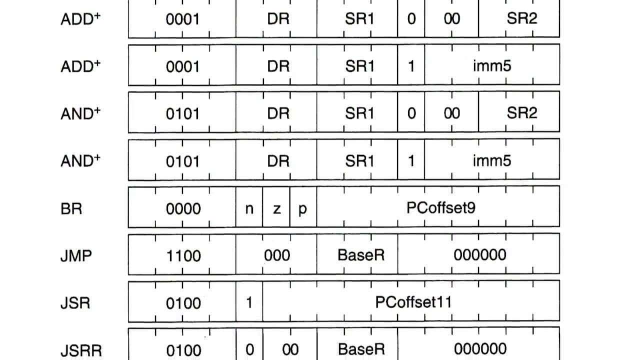 day, week and year, Then calculate any tax to be added, And so on. An informal high-level description of a program like this is called pseudocode. Then, when the program was all figured out on paper, they'd painstakingly expand and 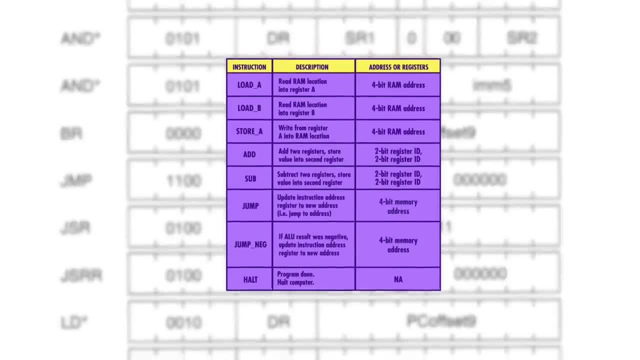 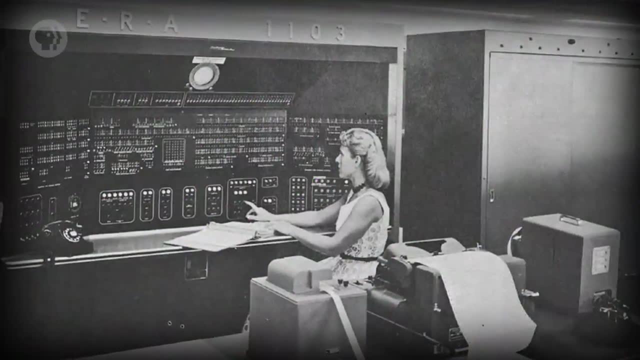 translate it into binary machine code by hand using things like opt code tables. After the translation was complete, the program could be fed into the computer and run. As you might imagine, people quickly got fed up with this process. So by the late 1940s and into the 50s, programmers had developed slightly higher-level languages. 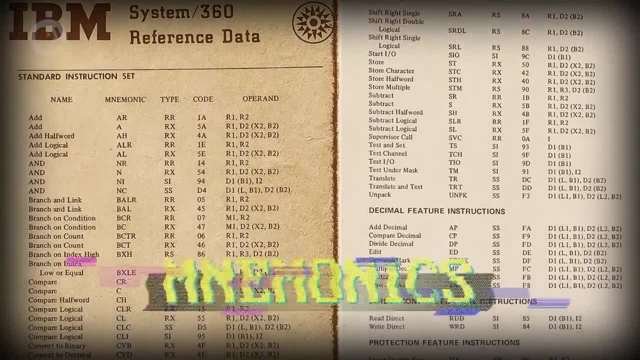 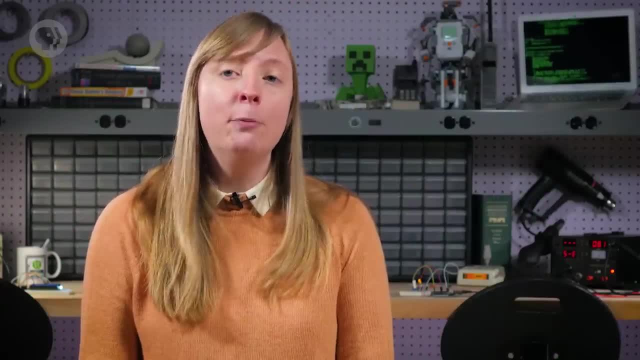 that were more human-readable. Opt code was the first language to be developed. The codes were given simple names called mnemonics, which were followed by operands to form instructions. So, instead of having to write instructions as bunches of 1s and 0s, programmers could. 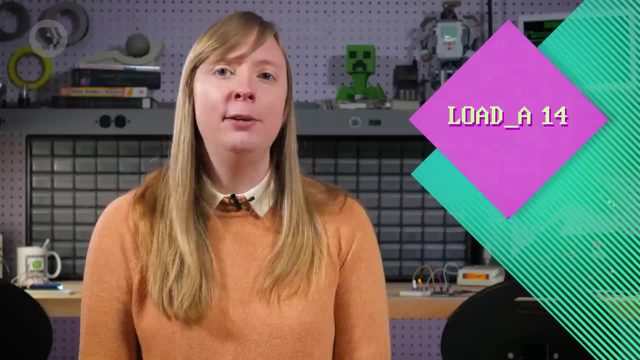 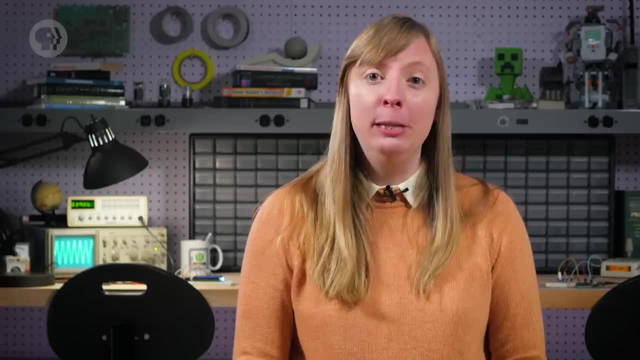 write something like Load A14.. We use this mnemonic in Episode 8 because it's so much easier to understand. Of course, a CPU has no idea what Load A14 is. It doesn't understand text-based language, only binary, And so programmers came up with a clever trick. 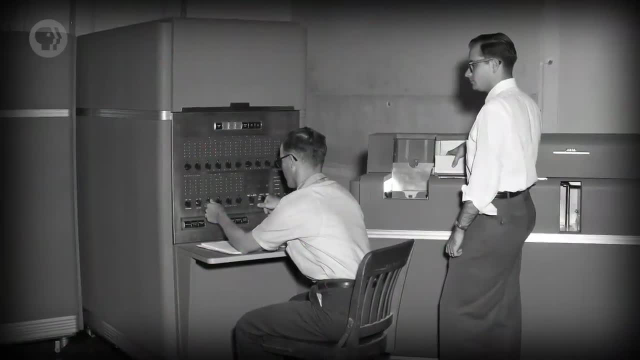 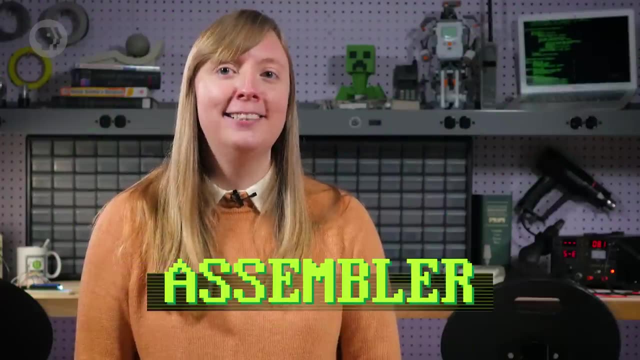 They created reusable helper programs in binary that read in text-based instructions and assemble them into the corresponding binary instructions automatically. This program is called- you guessed it- an assembler. It reads in a program written in an assembly language and converts it to native machine. 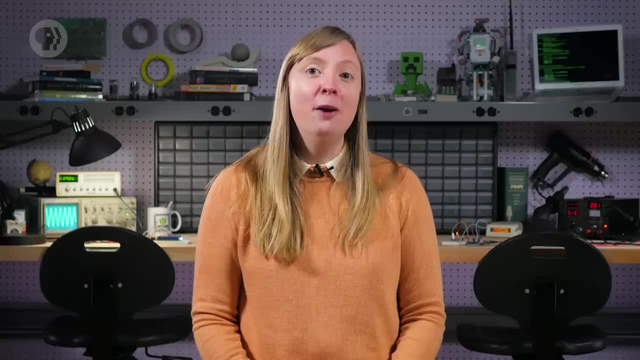 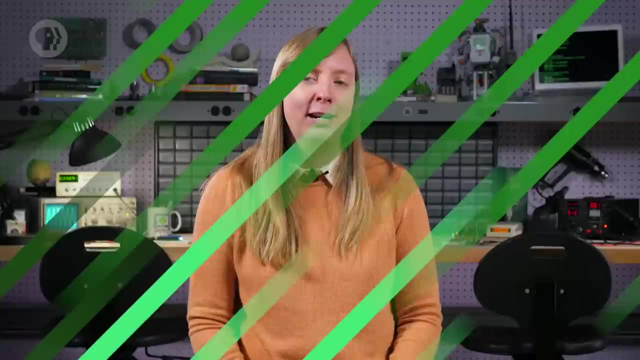 code Load A14 is one example of an assembly instruction. Over time, assemblers gained new features that made programming even easier. One nifty feature is automatically figuring out jump addresses. This was an example program I used in Episode 8.. 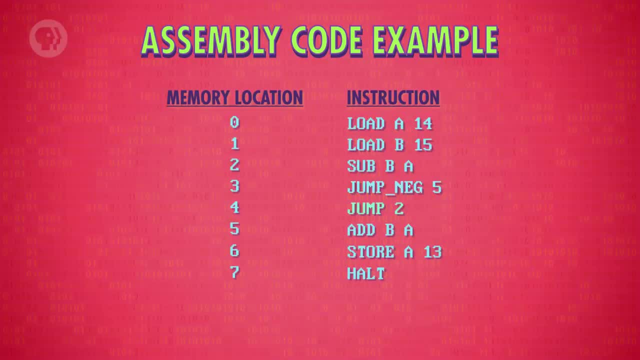 Notice how our jump negative instruction jumps to address 5, and our regular jump goes to address 2.. In other words, if we add more code to the beginning of this program, all of the addresses would change. That's a huge pain if you ever want to update your program. 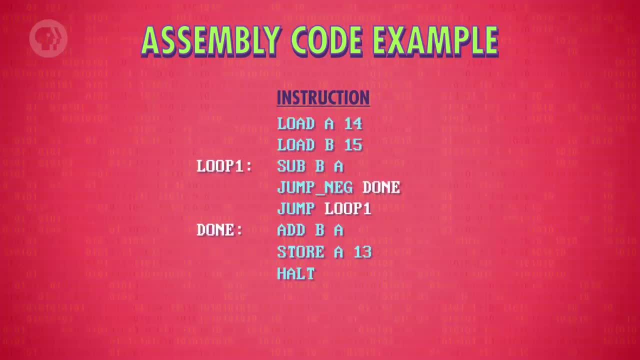 And so an assembler does away with raw jump addresses and lets you insert little labels that can be jumped to. When this program is passed into the assembler, it does the work of figuring out all of the jump addresses. Now the programmer can focus more on programming and less on the underlying mechanics. under 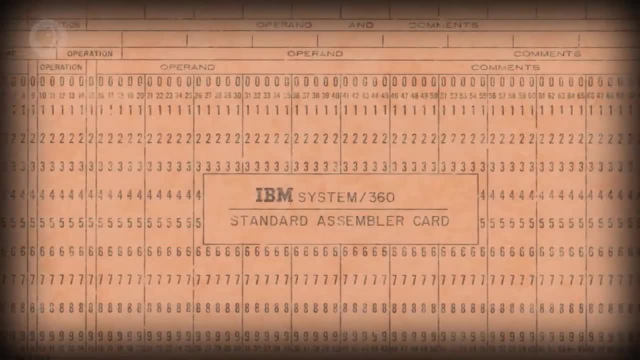 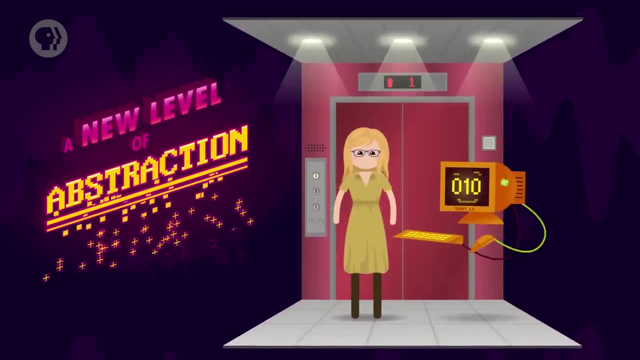 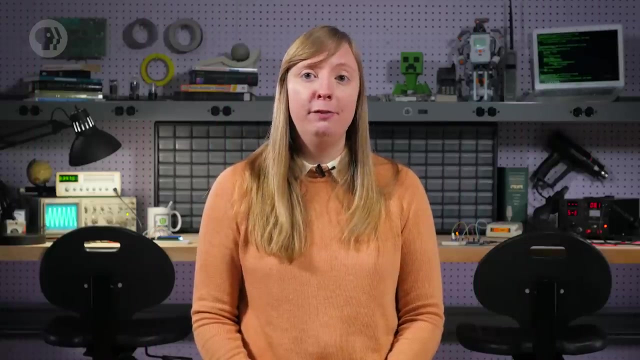 the hood, enabling more sophisticated things to be built, but hiding unnecessary complexity. As we've done many times in this series, we're once again moving up another level of abstraction. However, even with nifty assembler features like auto-linking, jumps to labels assembly. 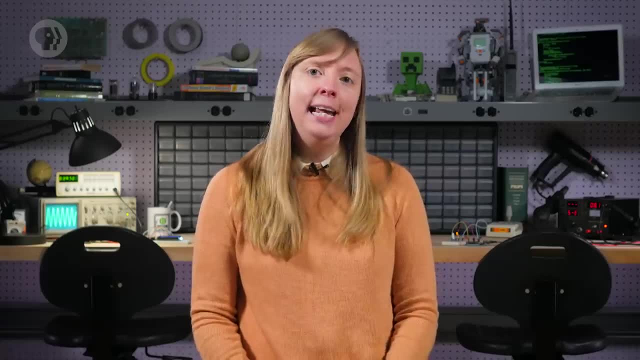 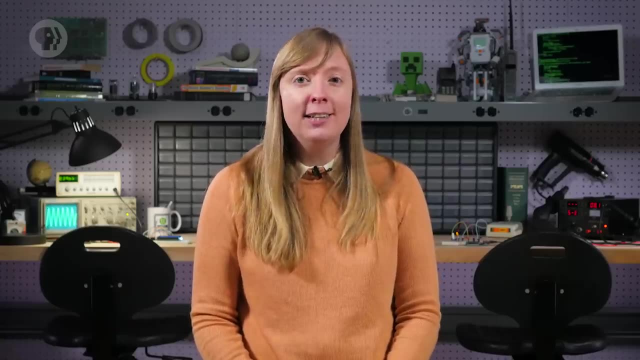 languages are still a thin veneer over machine code. In general, each assembly language instruction converts directly to a corresponding machine instruction – a one-to-one mapping – so it's inherently tied to the underlying hardware, And the assembler still forces programmers to think about which registers and memory. 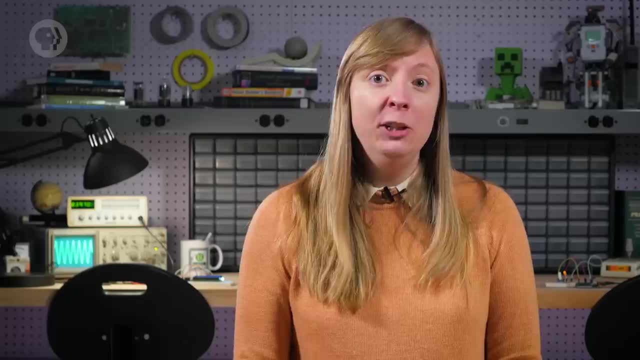 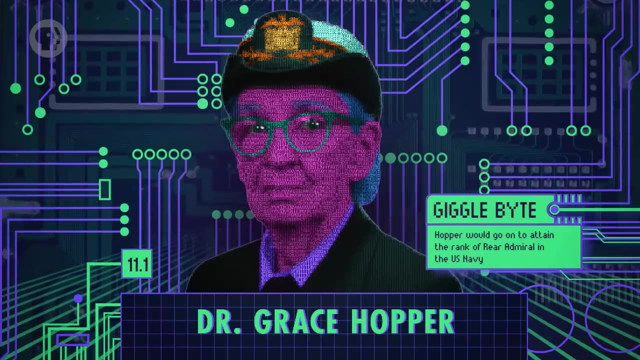 locations they will use. If you suddenly needed an extra value, you might have to do a little bit more work on it. Let's go to the thought bubble. This problem did not escape Dr Grace Hopper. As a US Naval officer, she was one of the first programmers on the Harvard Mark I computer. 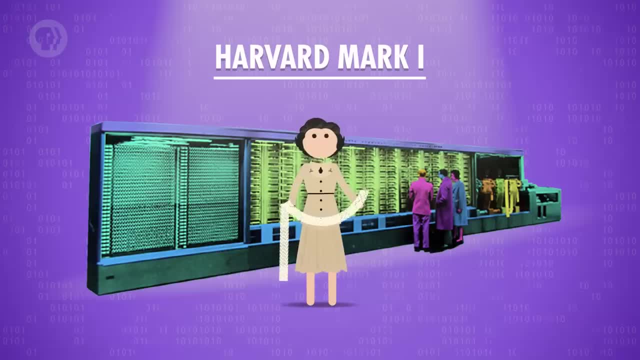 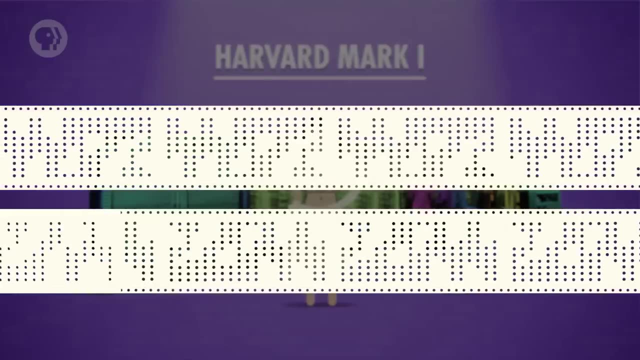 which we talked about in Episode 2.. This was a colossal electro-mechanical beast, completed in 1944 as part of the Allied war effort. Programs were stored and fed into the computer on punch paper tape. By the way, as you can see, they patched some bugs in this program by literally putting 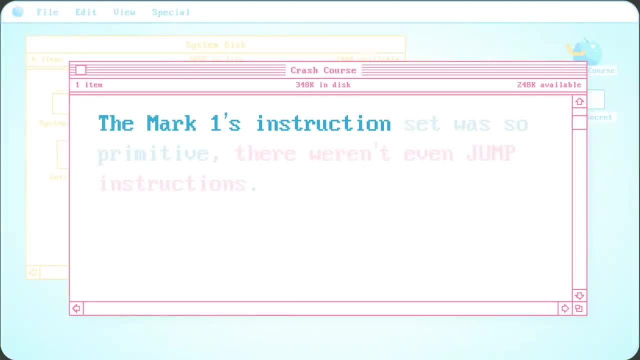 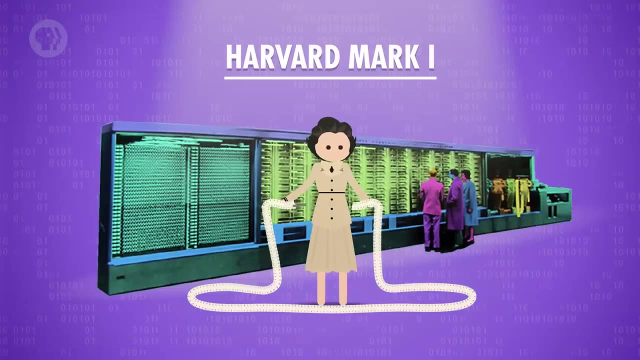 patches of paper over the holes on the punch tape. The Mark I's instructions are as follows. The first instruction set was so primitive there weren't even jump instructions To create code that repeated the same operation multiple times. you'd tape the two ends. 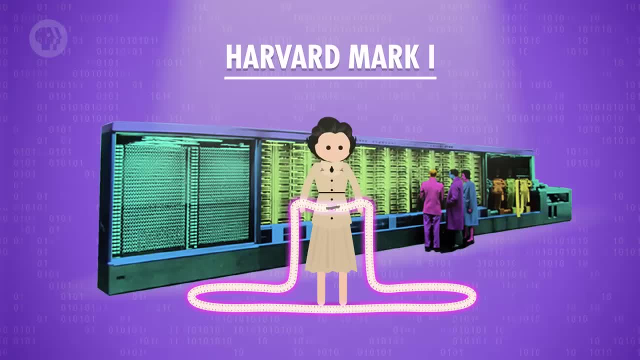 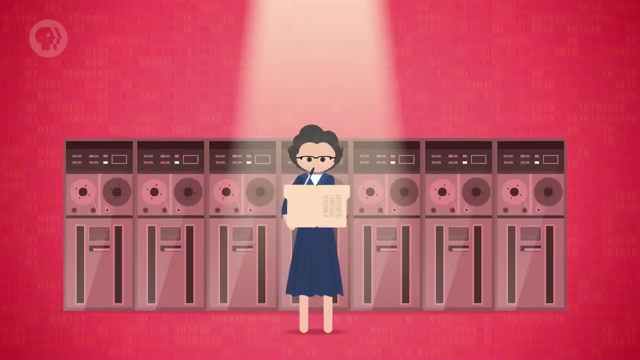 of the punch tape together, creating a physical loop, In other words programming the Mark. I was kind of a nightmare. After the war. Hopper continued to work at the forefront of computing To unleash the potential of computers. she designed a high-level programming language. 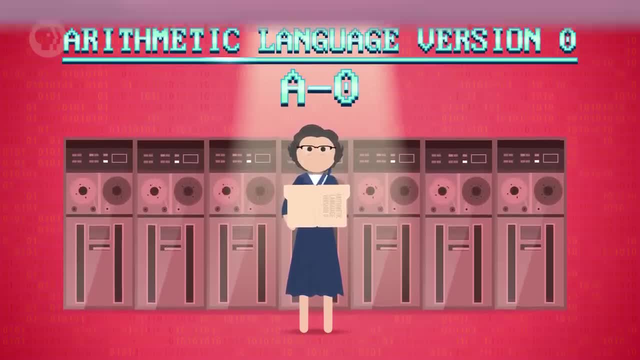 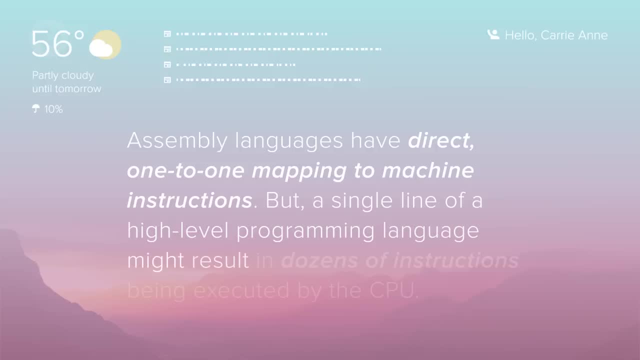 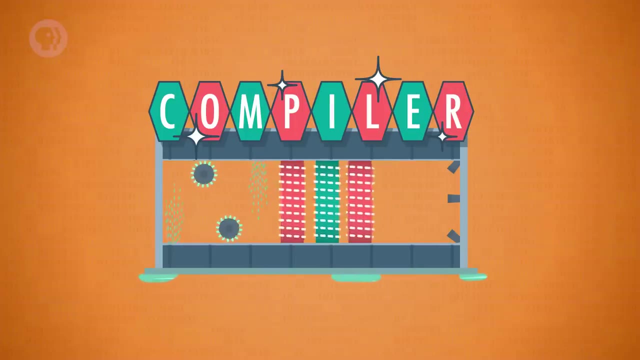 called Arithmetic Language Version Zero, or A0 for short. Assembly languages have direct one-to-one mapping-to-machine instructions, but a single use of a high-level programming language might result in dozens of instructions being executed by the CPU To perform this complex translation. Hopper built the first compiler in 1952.. 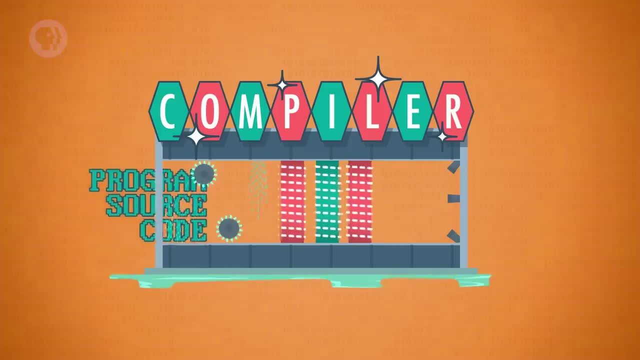 This is a specialized program that transforms source code written in a programming language into a low-level language like assembly or the binary machine code that the CPU can directly process. Thanks, Thought Bubble. So, despite the promise of easier programming, many people were skeptical of Hopper's idea. 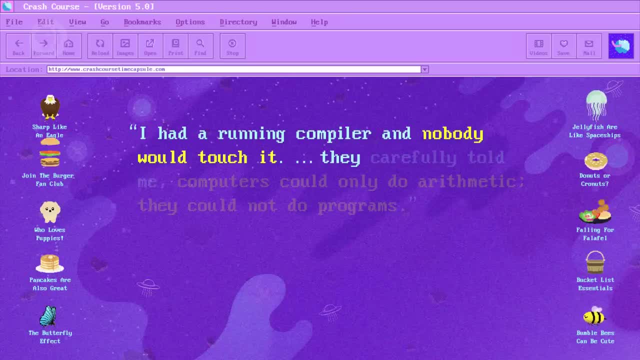 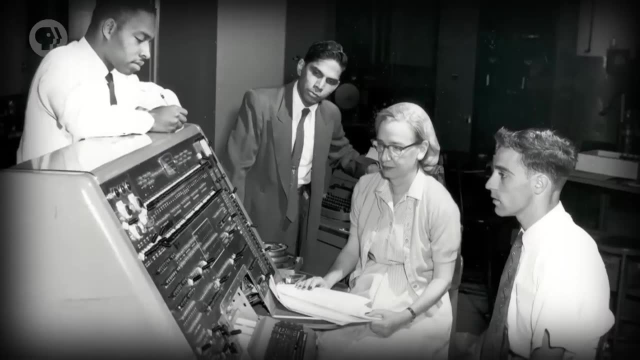 She once said, I had a running compiler and nobody would touch it. They carefully told me computers could only do arithmetic, they could not do programs. But the idea was a good one, and soon many efforts were underway to craft new programming. 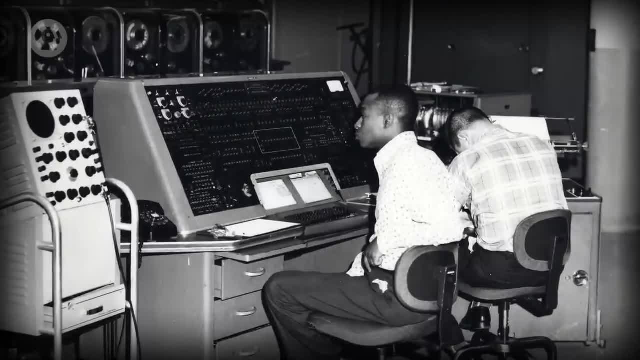 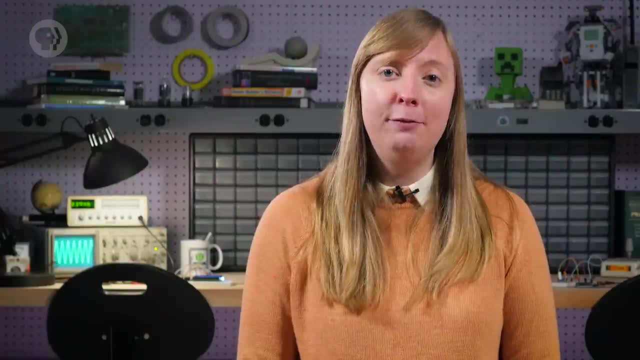 languages Today there are hundreds. Sadly, there are no surviving examples of A0 code, so we'll use Python, a modern programming language, as an example. Let's say we want to add two numbers and save the value. Remember in assembly code we had to fetch values from memory, deal with registers and 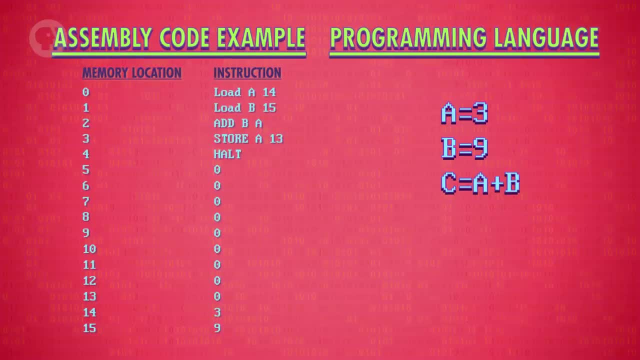 other low-level details. But this same program can be written in Python like so. Notice how there are no registers on the code. The compiler takes care of that stuff, abstracting away a lot of low-level and unnecessary complexity. The programmer just creates abstractions for needed memory locations, known as variables. 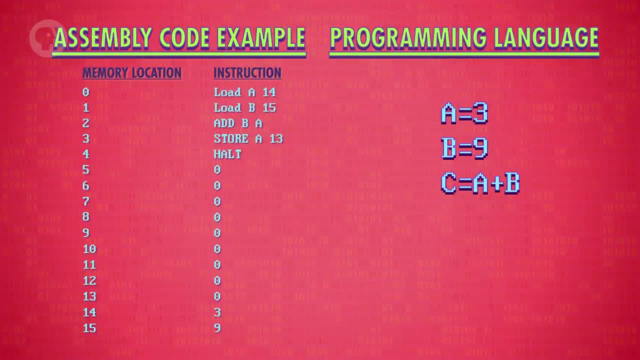 and gives them names. So now we can just take our two numbers, store them in variables we give names to- In this case I picked A and B, but those variables could be anything- and then add those together, saving the result in C, another variable I created, 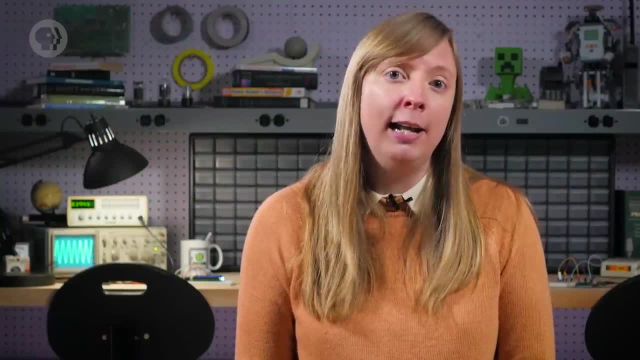 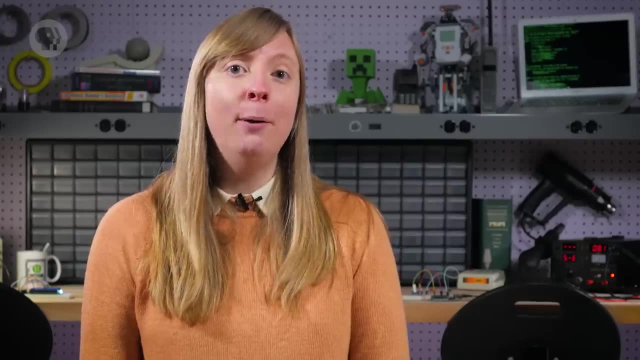 It might be that the compiler assigns register A under the hood to store the value in A, but I don't need to know about it Out of sight, out of mind. It was an important historical milestone, but A0 and its later variants weren't widely. 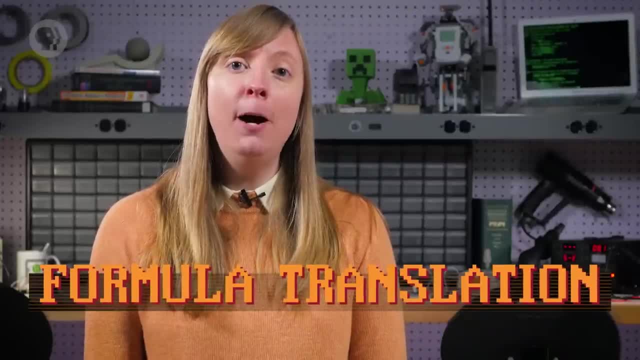 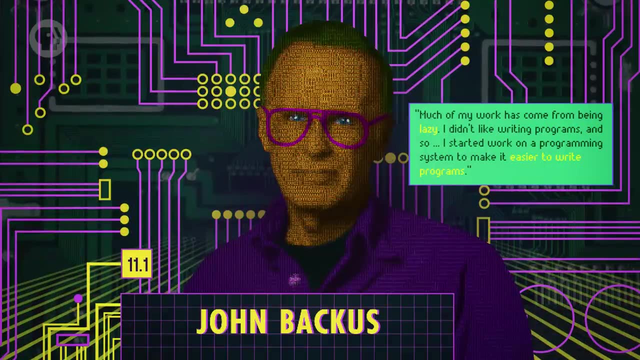 used. FORTRAN, derived from formula translation, was released by IBM a few years later, in 1957, and came to dominate early computer programming. John Backus, the FORTRAN project director, said: Much of my work has come from being lazy. 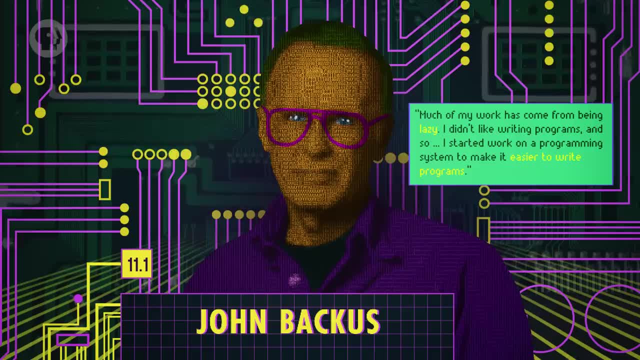 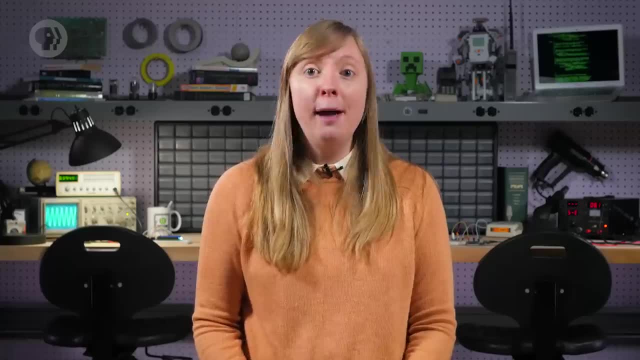 I didn't like writing programs, and so I started work on a programming system to make it easier to write programs. You know, typical lazy person. Anyway, on average, programs written in FORTRAN were 20 times shorter than equivalent handwritten assembly code. Then the FORTRAN compiler would translate and expand that into native machine code. The community was skeptical that the performance would be as good as handwritten code, but the fact that programmers could write more code more quickly made it an easy choice economically trading a small increase in computation time for a significant decrease in programmer time. 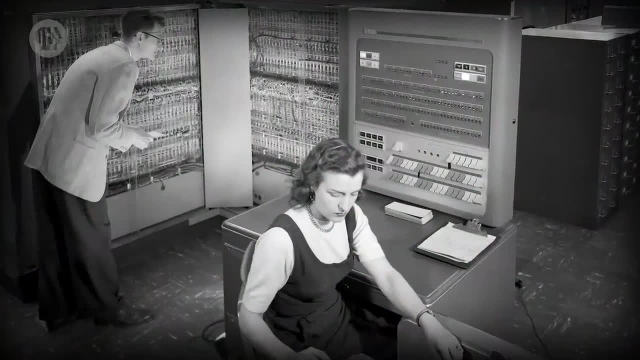 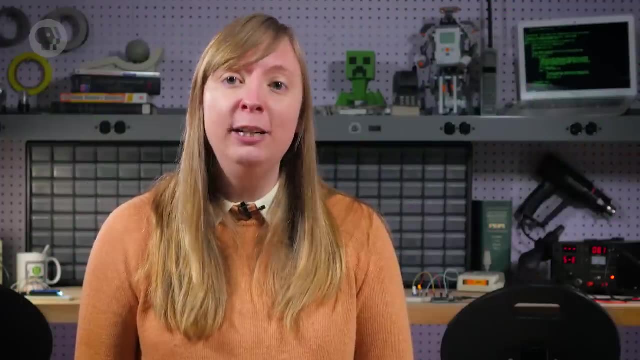 Of course IBM was in the business of selling computers, and so initially FORTRAN code could only be compiled and run on IBM computers, And most programming languages and compilers of the 1950s could only run on a single type of computer. 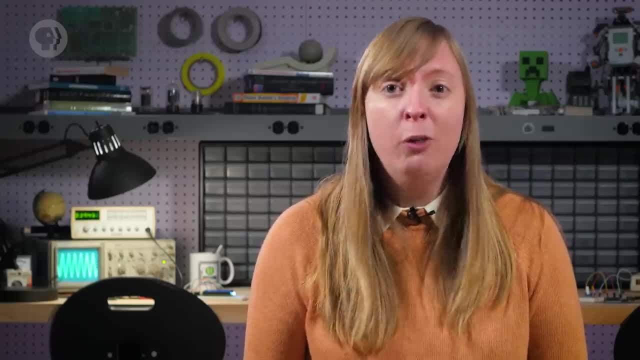 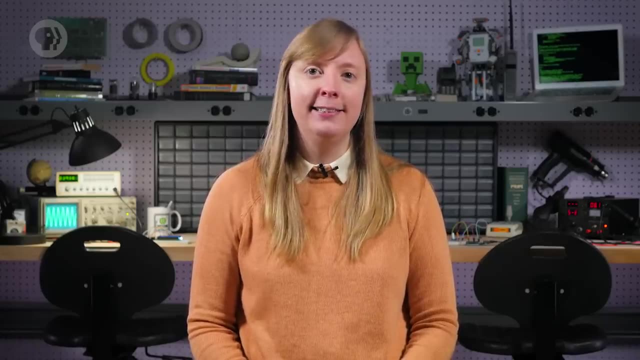 So if you upgraded your computer you'd often have to rewrite all the code too. In response, computer experts from industry, academia and government formed a consortium in 1959, the Committee on Data Systems Languages, advised by our friend Grace Hopper to guide. 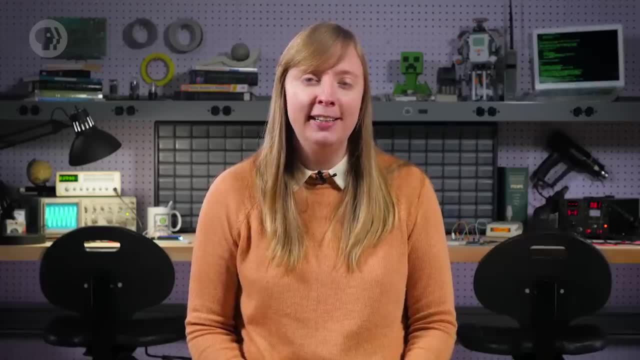 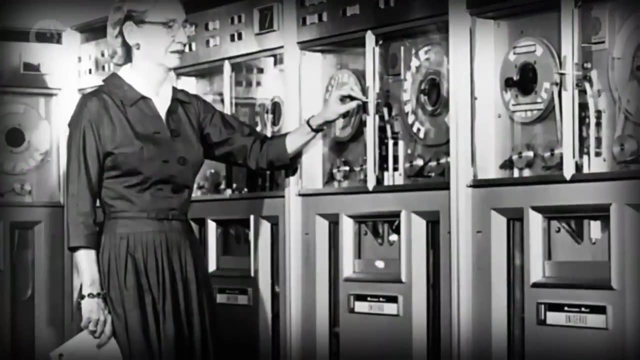 the development of a common programming language that could be used across different machines. The result was the high-level, easy-to-use common business-oriented language, or COBOL for short. For example, for hardware, each computing architecture needed its own COBOL compiler. 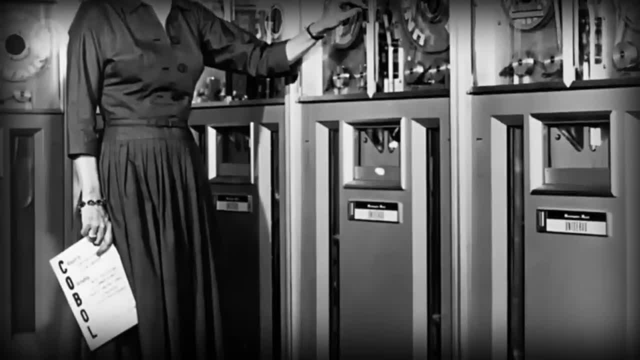 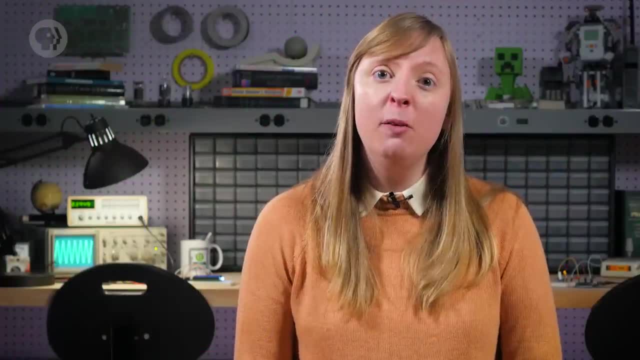 But critically, these compilers could all accept the same COBOL source code, no matter what computer it was run on. This notion is called Write Once, Run Anywhere. It's true of most programming languages today. a benefit of moving away from assembly. 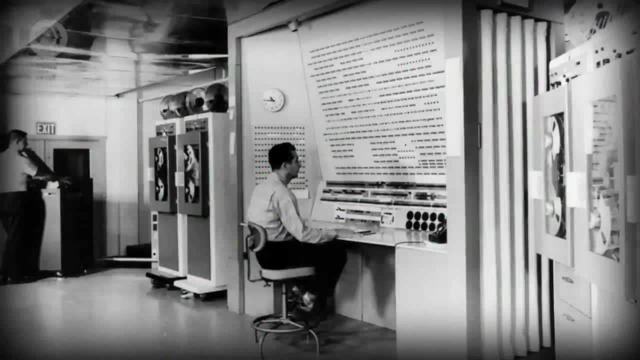 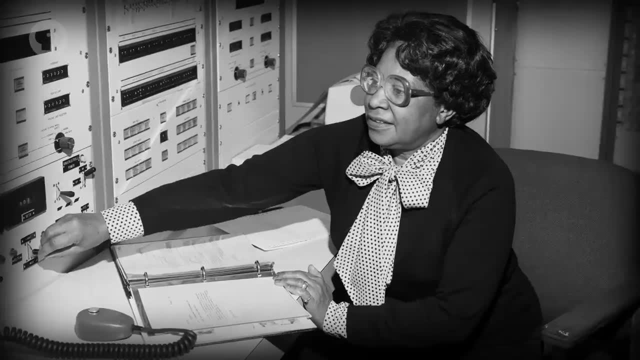 and machine code which is still CPU-specific. The biggest impact of all of this was reducing computing's barrier to entry. Before high-level programming languages existed, it was the realm exclusive to computer experts and enthusiasts, And it was often their full-time profession. 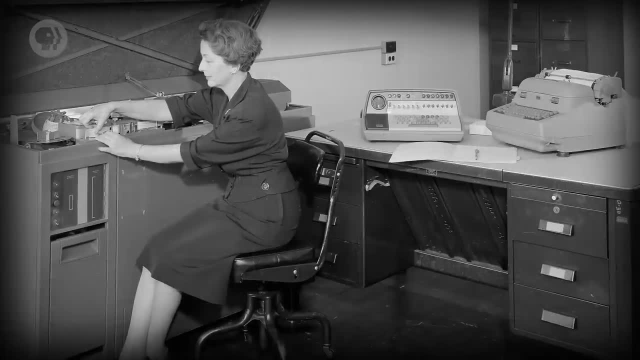 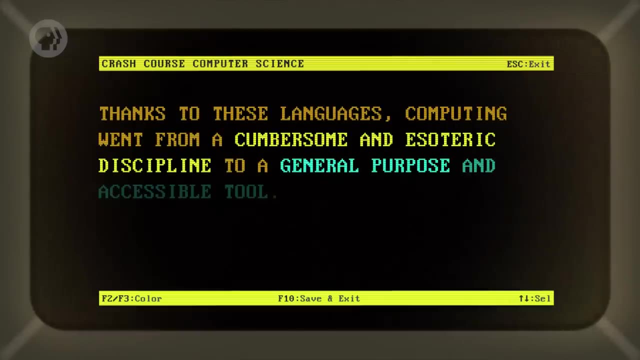 Scientists, engineers, doctors, economists, teachers and many others could incorporate computation into their work. Thanks to these languages, computing went from a cumbersome and esoteric discipline to a general-purpose and accessible tool. At the same time, abstraction in programming allowed those computer experts now professional. 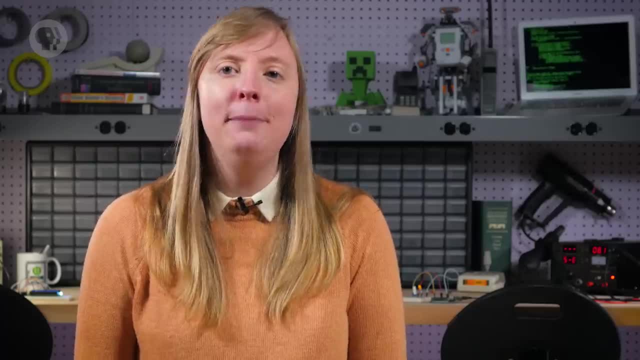 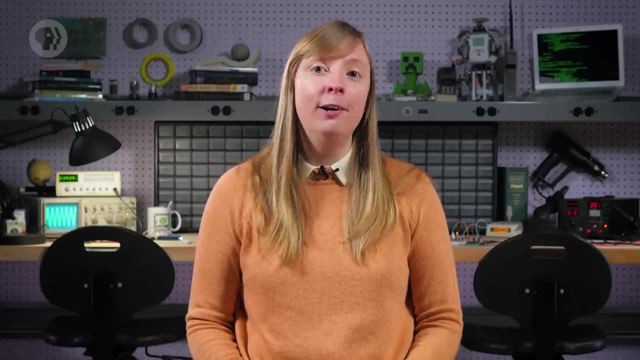 programmers to create increasingly sophisticated programs which would have taken millions, tens of millions or even more lines of assembly code. Now, this history didn't end in 1959. In fact, a golden era in programming language design jump-started. 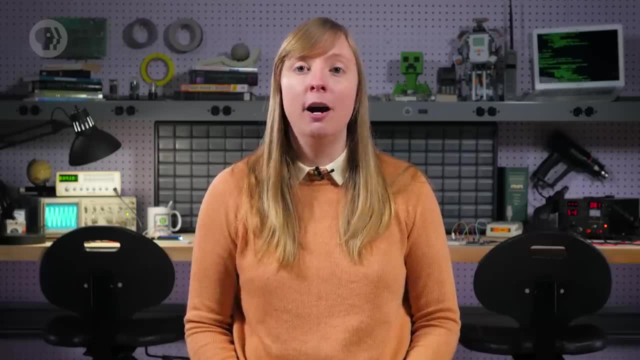 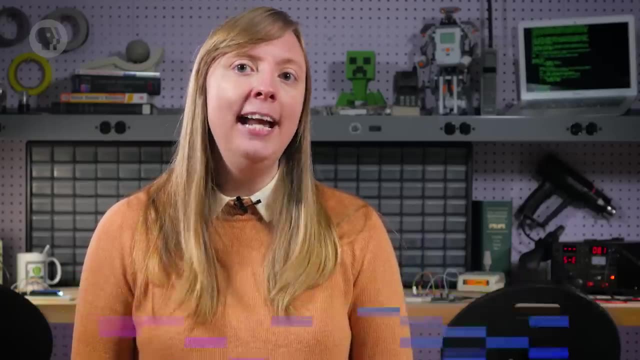 It started in the 1950s. It started in lockstep with dramatic advances in computer hardware. In the 1960s we had languages like ALGO, LISP and BASIC. In the 70s, Pascal, C and Smalltalk were released. 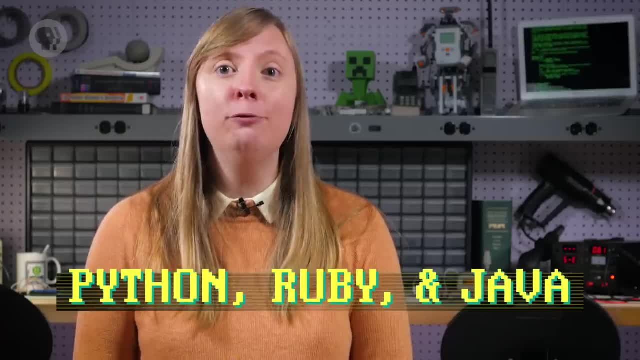 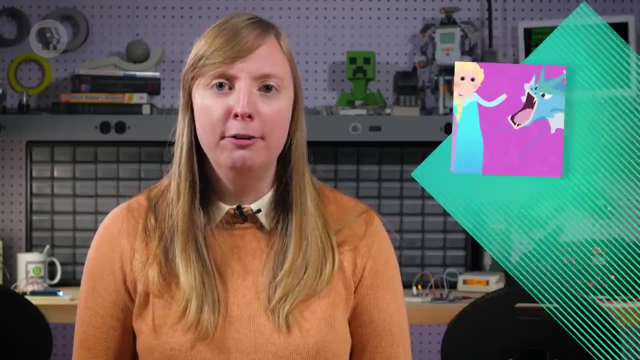 The 80s gave us C++, Objective-C and Perl, And the 90s Python, Ruby and Java. And the new millennium has seen the rise of Swift, C-Sharp and Go- Not to be confused with Let It Go and Pokemon Go. 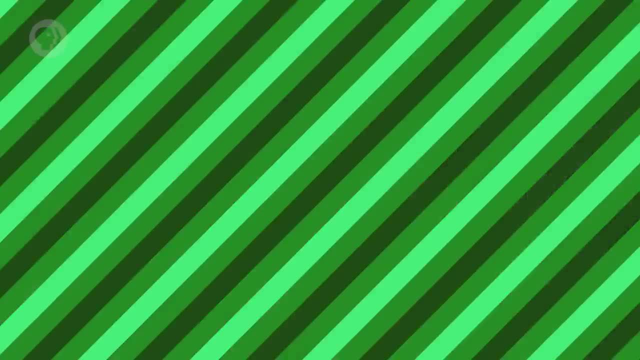 Anyway, some of these might sound familiar. Many are still around today. It's extremely likely that the web browser you're using right now was written in C++ or Objective-C. That list I gave is just the beginning. I hope you enjoyed this video. 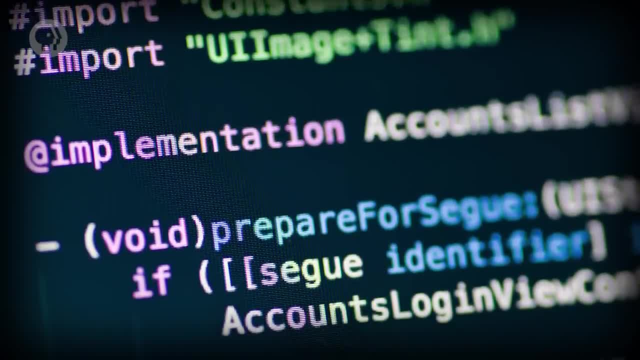 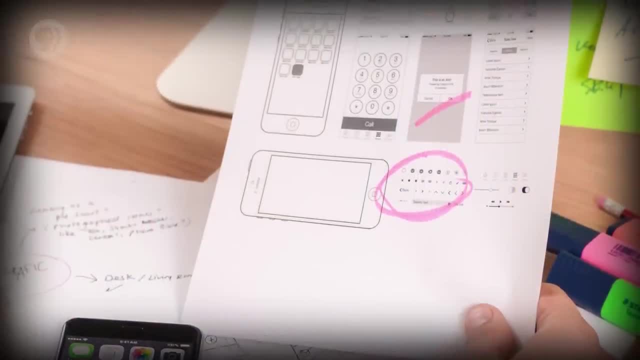 This is the tip of the iceberg, and languages with fancy new features are proposed all the time. Each new language attempts to leverage new and cleverer abstractions to make some aspect of programming easier or more powerful, or take advantage of emerging technologies and platforms so that more people can do more amazing things more quickly. 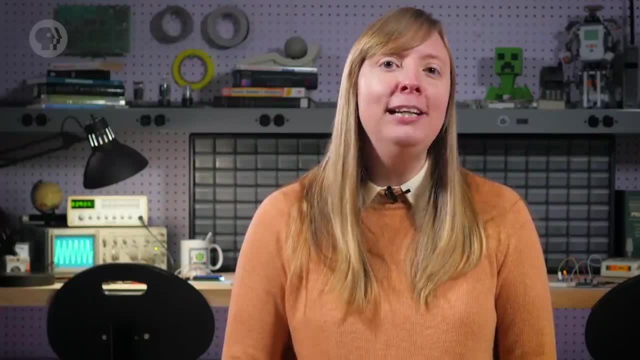 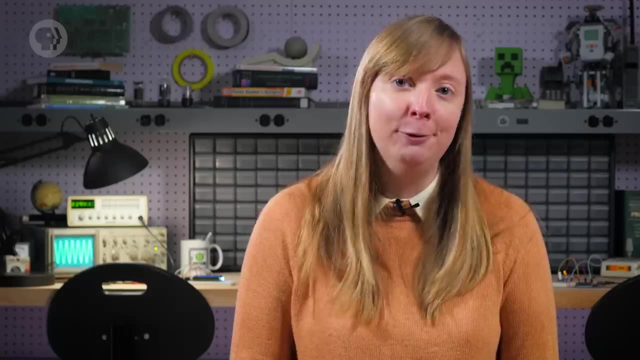 Many consider the holy grail of programming to be the use of plain old English, where you can literally just speak what you want the computer to do. it figures it out and executes it. This kind of intelligent system is science fiction for now. 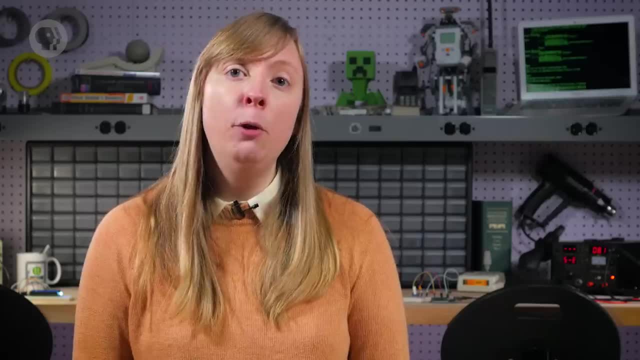 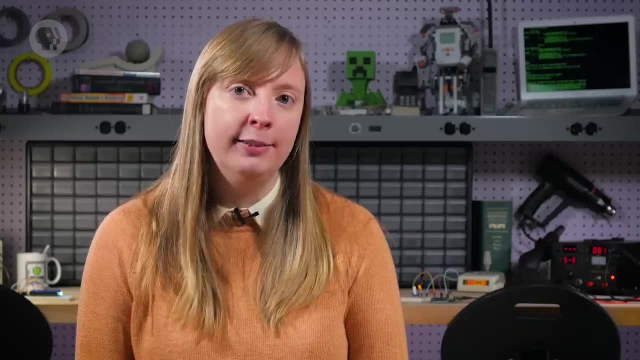 And fans of 2001 A Space Odyssey may be OK with that. If you want to know all about programming languages, we're going to deep-dive for the next couple of episodes and we'll continue to build your understanding of how programming languages and the software they create are used to do cool and unbelievable things. 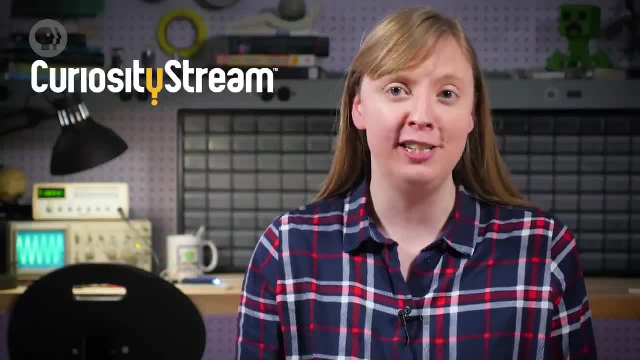 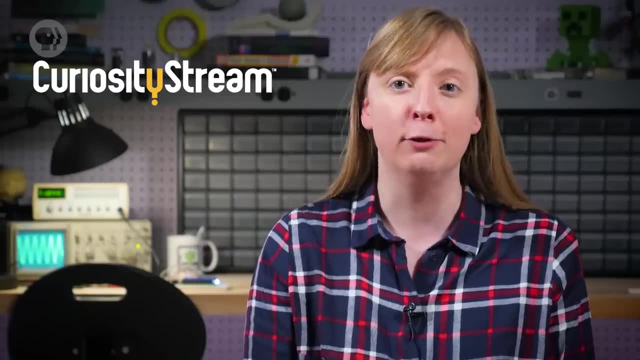 See you next week. Hey guys, this week's episode was brought to you by CuriosityStream, which is a streaming service full of documentaries and non-fiction titles for some really great filmmakers, including exclusive originals. I just watched a great series called Digits, hosted by our friend Derek Mueller. 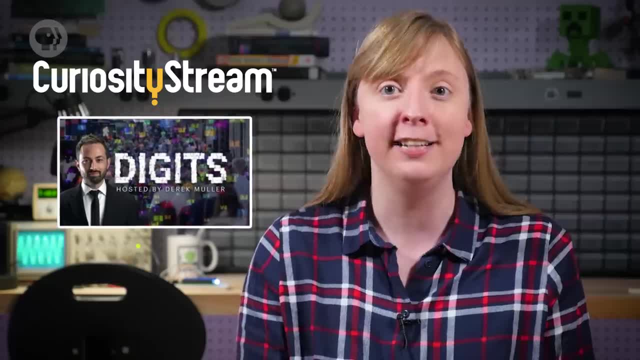 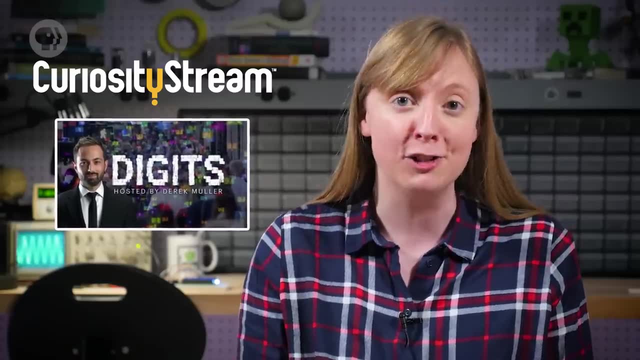 It's all about the internet, From the origins to the proliferation of the Internet of Things, to ethical or white-hat hacking, And it even includes some special guest appearances, like that John Green guy you keep mentioning in the comments. And CuriosityStream offers unlimited access starting at $2.99 a month. 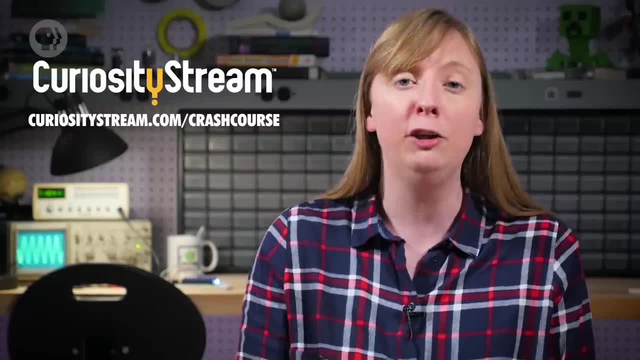 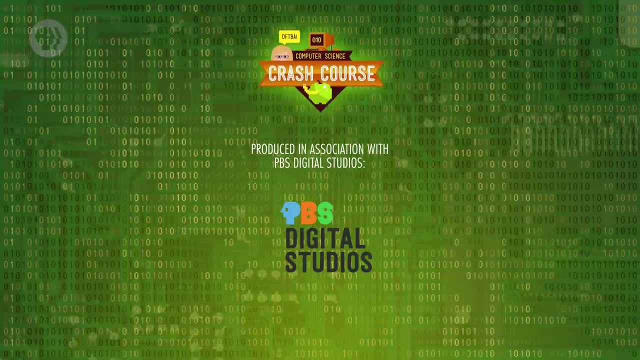 And for you guys, the first two months are free if you sign up at curiositystreamcom. slash crashcourse and use the promo code CRASHCOURSE during the sign-up process. Crash Course- Computer Science is produced in association with PBS Digital Studios. 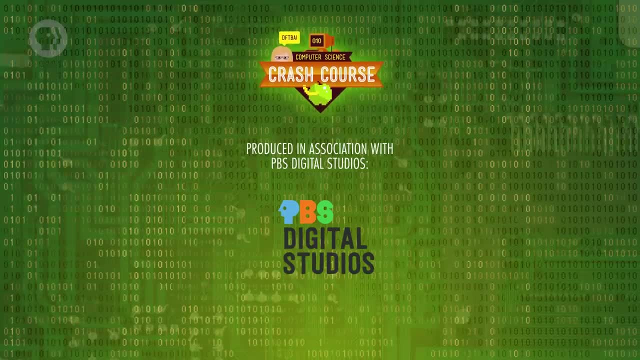 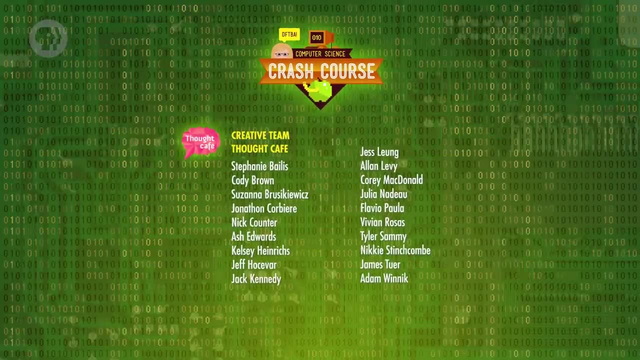 Like their channel. you can check out a playlist of shows like Gross Science, ACS Reactions and The Art Assignment. This episode was filmed at the Chad and Stacey Emigolch Studio in Indianapolis, Indiana, And it was made with the help of all these nice people and our wonderful graphics team. 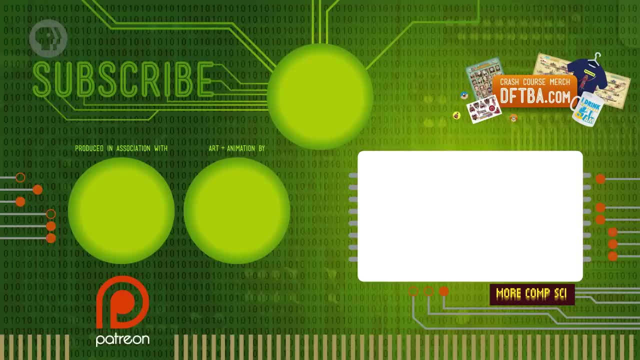 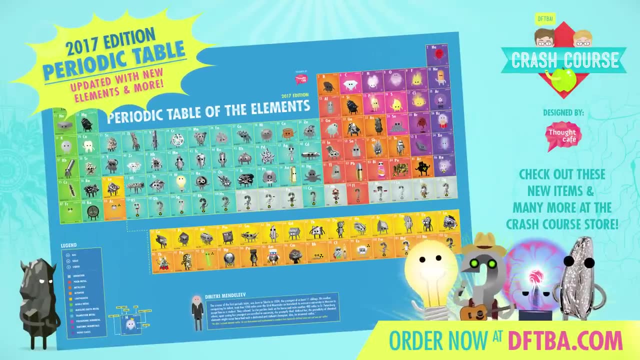 Thought Cafe. Thanks for watching and try turning it off and then back on again. Subtitles by the Amaraorg community.